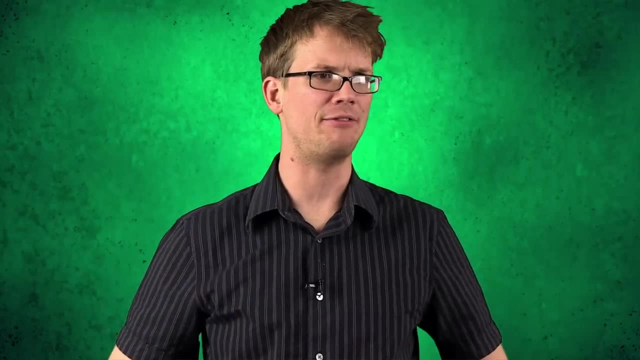 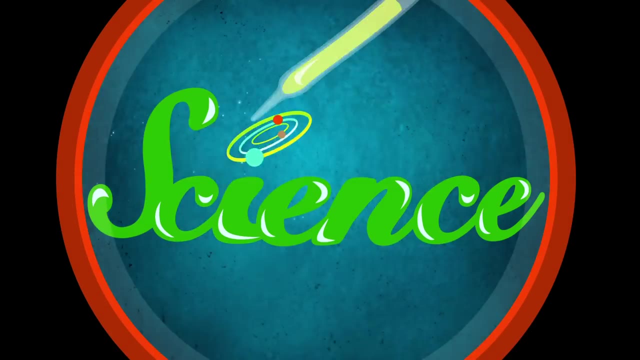 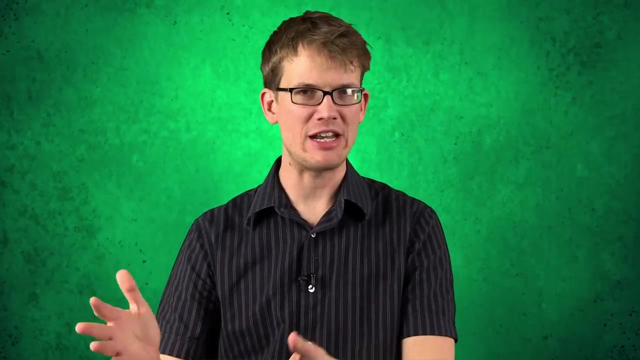 to be wonderful for making a whole class of new words that will have abilities that no word has ever had before. Everybody welcome to the world of chemistry. So a chemical element is a substance with a particular set of properties that can't be broken down any further than it's already been broken down. Elements are the building. 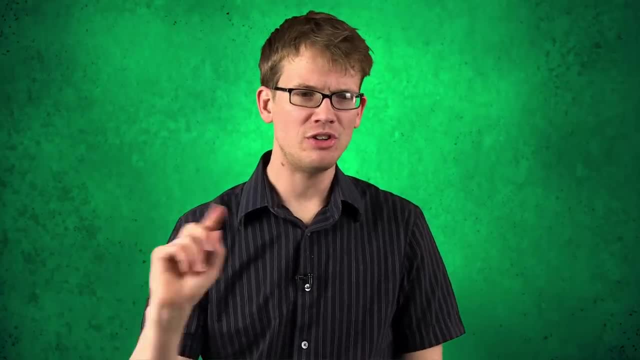 blocks of matter. They are the chemist's alphabet, But unlike the alphabet, which is completely arbitrary, why does it go? A, B, C, D, E, F, G, I, T? who knows Who did that? 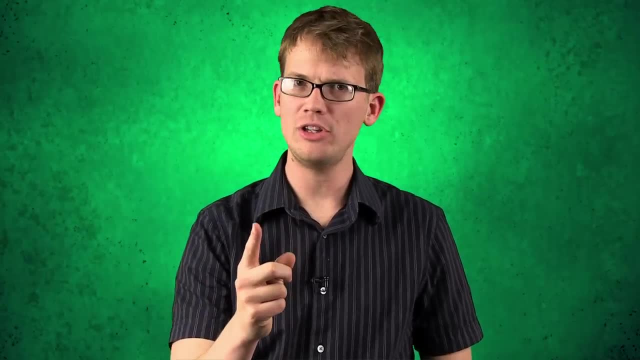 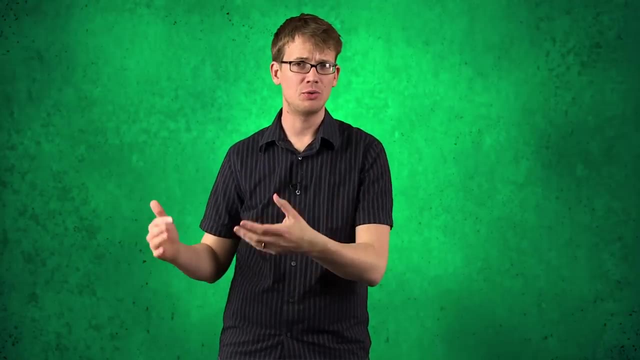 It doesn't have to go in that order. Elements are actually set by laws of the universe, So sometimes, even recently, we've been able to create new ones. In 2011,, we finally got around to naming them, So we started naming some elements that were created in the 1990s. Welcome to Copernicium. 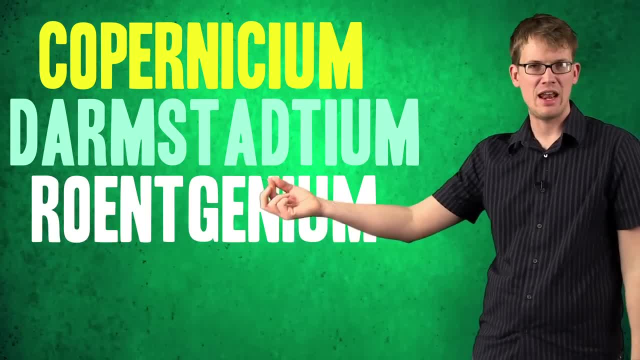 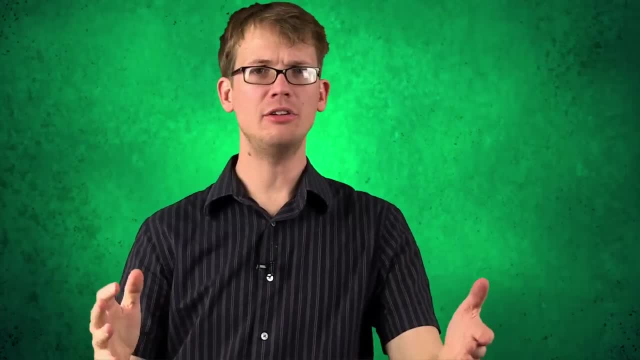 Also Darmstadium And Rot-Gnenny- I don't know how to pronounce that one- Anybody. So we've got now 118 elements which either just exist on the Earth or have been created in a laboratory And, unsurprisingly, it took some doing to get a system together that could. 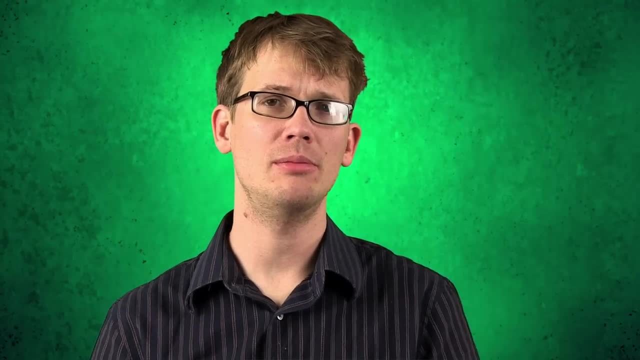 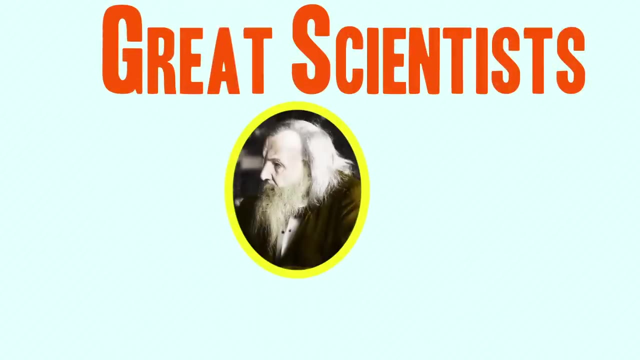 organize all of that stuff pretty well. But creating a system to organize all of these elements is exactly what Dmitri Ivanovich Mendeleev did- And yeah, he was a Russian dude. Obviously, this guy was built for science, But not necessarily more so than this guy, Or this guy Or this. 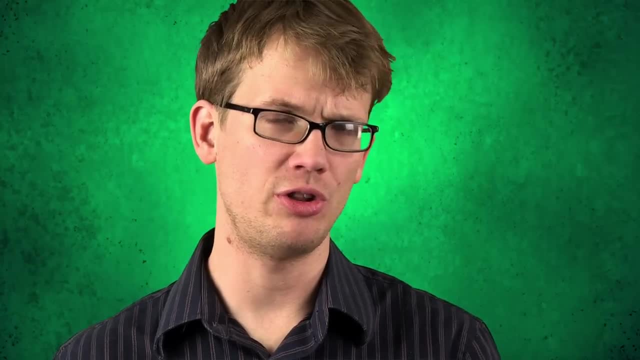 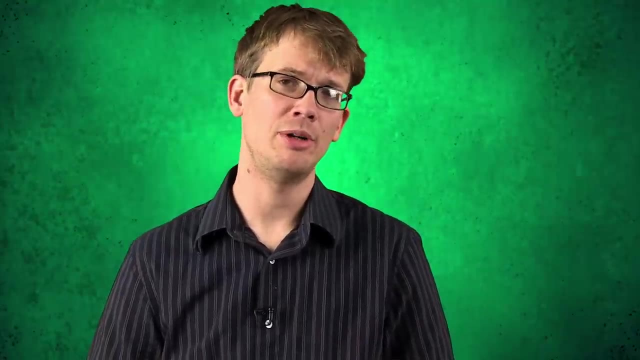 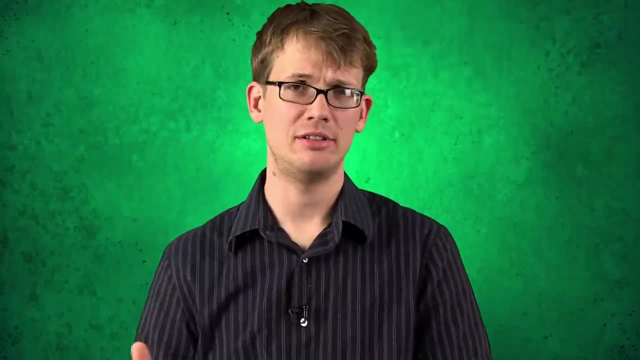 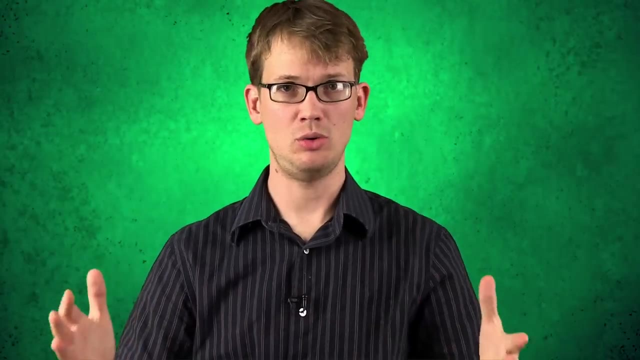 after him and you don't. In Mendeleev's day only about 60 elements existed, And he really needed some money, so he was writing a chemistry textbook. But he needed a way to organize all of these elements into a table, So he decided: why not sort them by weight, From lightest to heaviest? 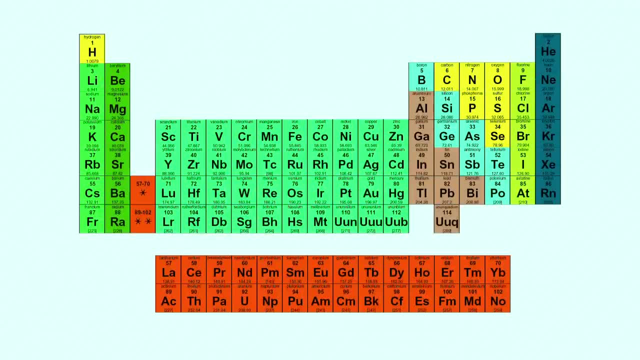 So Mendeleev started arranging elements into horizontal rows by atomic weight, But he fridged it a little bit to sort elements so that ones with similar physical properties were grouped together. But when he did this, a definite pattern started to suggest itself, But only.